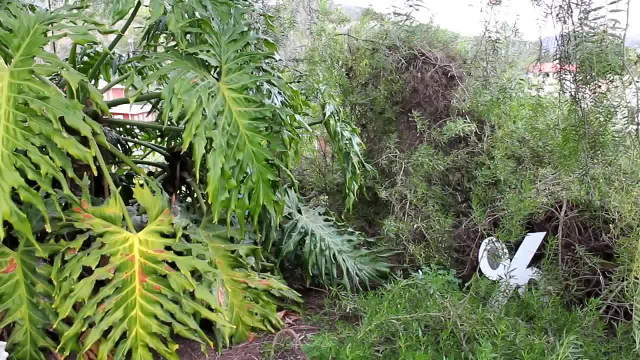 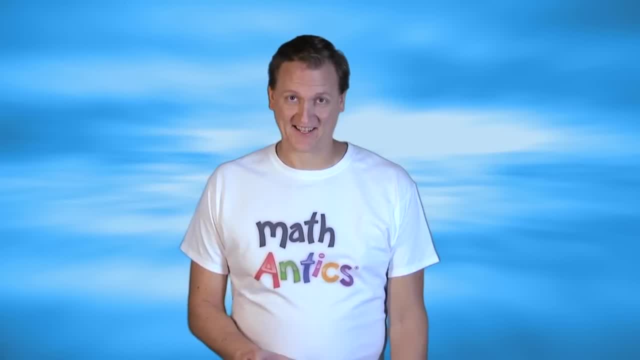 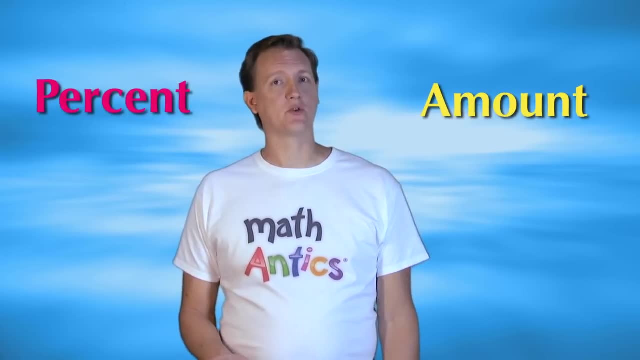 and then we have to go looking for them like a game of hide and seek Gotcha. Ummm… not exactly. Finding a percent of a number makes more sense if you remember that a number just represents an amount and that a percent is really just a fraction. 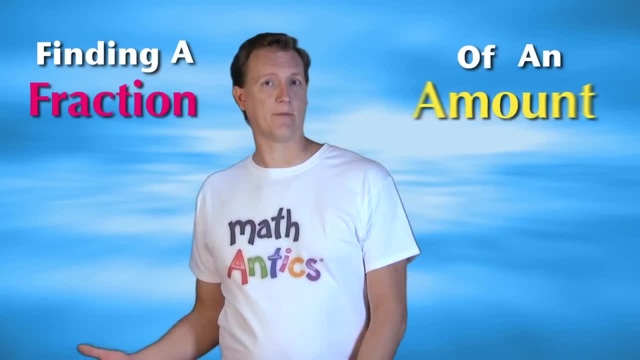 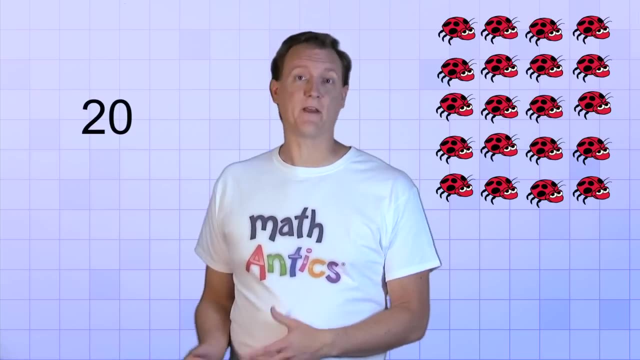 So finding a percent of a number really means finding a fraction of an amount. Think about it this way. Let's say, the number 20 represents an amount like the amount of ladybugs that you found at the park one day, And let's also imagine that you agreed to. 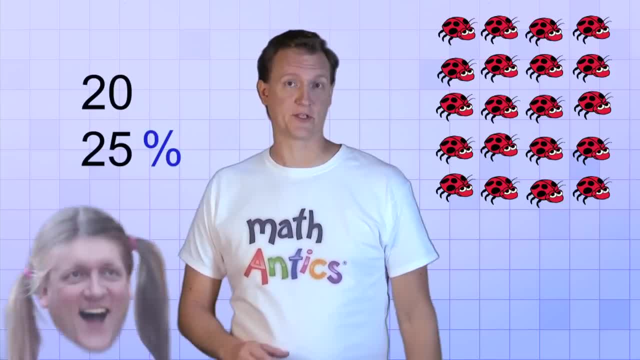 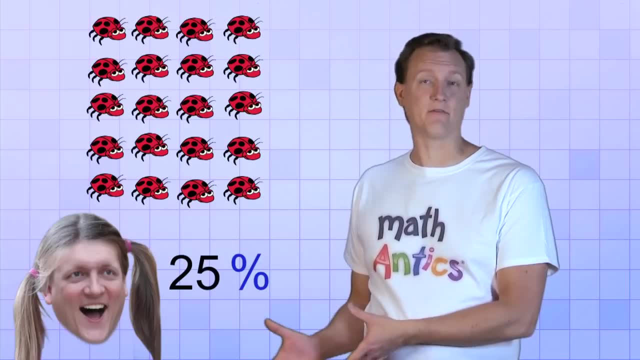 give 25% of all the ladybugs you found to your little sister. Okay then, so how many is that? If you have 20 ladybugs, how many is 25% of that amount? That's what it means: to find the percent of a number. 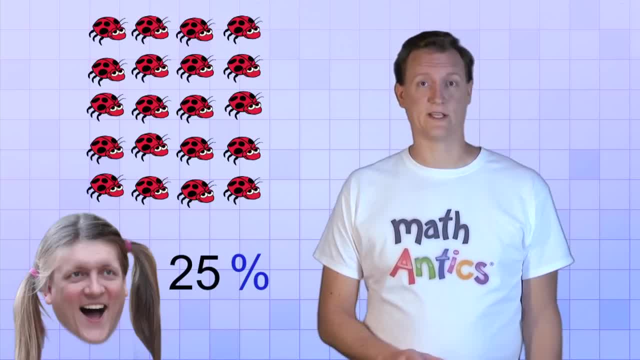 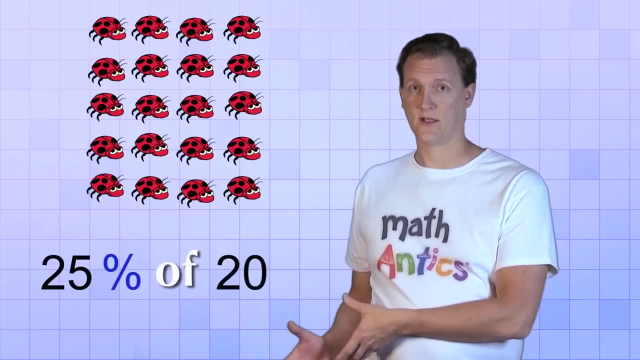 You're finding out how much that percent of the total is. In this case, since our total is 20, we need to know what 25% of 20 is. So how do we figure that out? Well, it's really easy, if you remember back to one of our fractions videos. 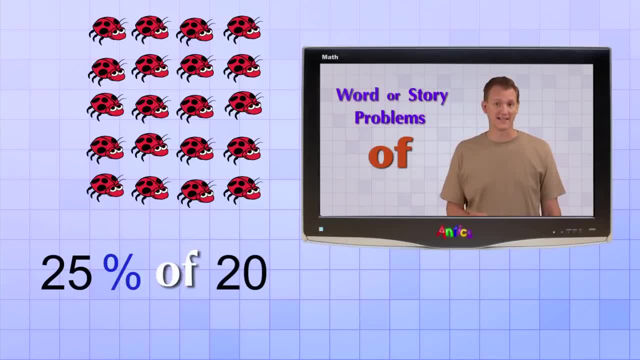 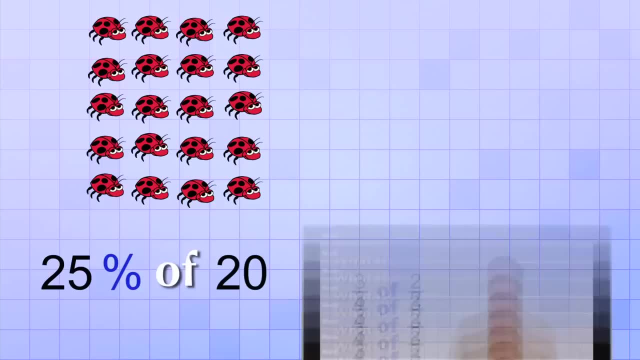 the one about multiplying fractions. In that video we learned that when dealing with fractions, sometimes the word OF is used instead of the multiplication symbol. When they say find one half of 16, they really mean find one half times 16.. 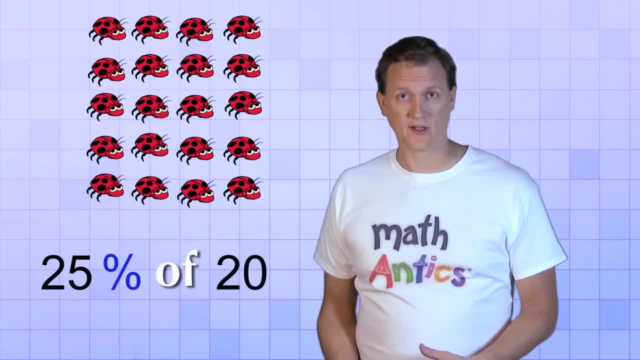 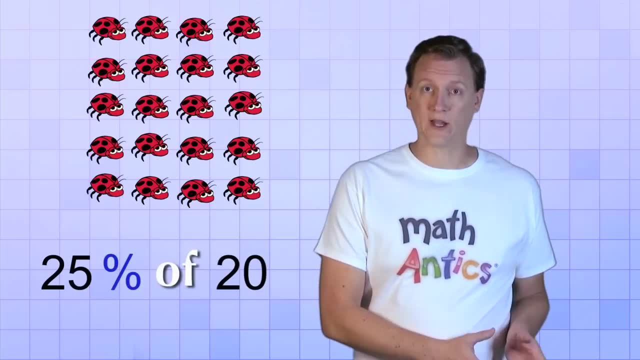 Well, guess what, Since a percent is just a special fraction OF, means the exact same thing with percents that it did with fractions. When we have 25% of 20,, that means the same as 25% times 20. Great. 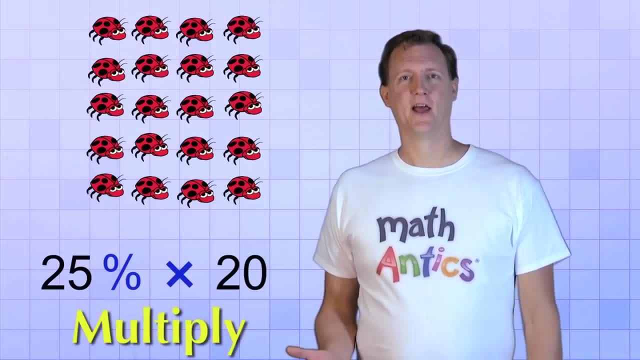 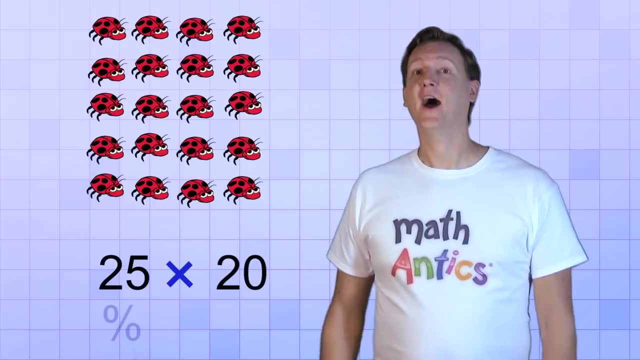 So all we have to do to find a percent of a number is to multiply. But how do we multiply a percent and a number together? Do we just forget about the percent sign and multiply the numbers together? No, If we did it that way, our number would be WAY too big. 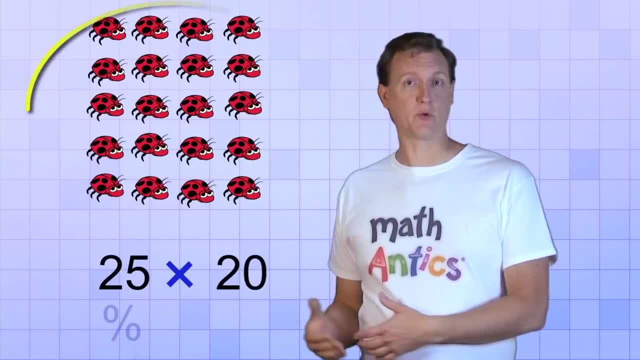 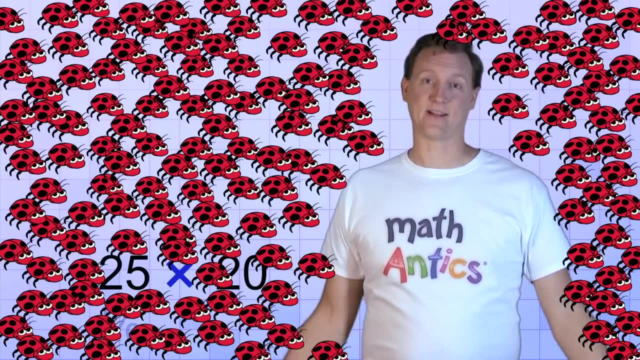 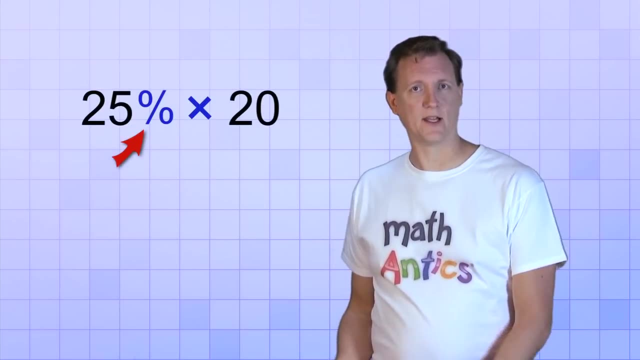 25% should be a smaller part of 20 ladybugs. But if we did 25 times 20, we'd get 500 ladybugs. Clearly that's not the right answer. Here's what we have to do instead. Remember that when you see a percent written like this, with the percent sign, 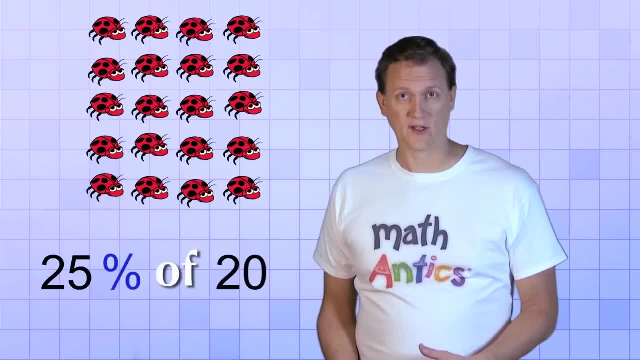 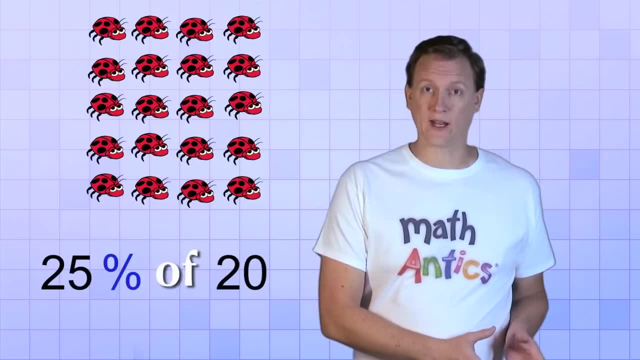 Well, guess what, Since a percent is just a special fraction OF, means the exact same thing with percents that it did with fractions. When we have 25% of 20,, that means the same as 25% times 20.. 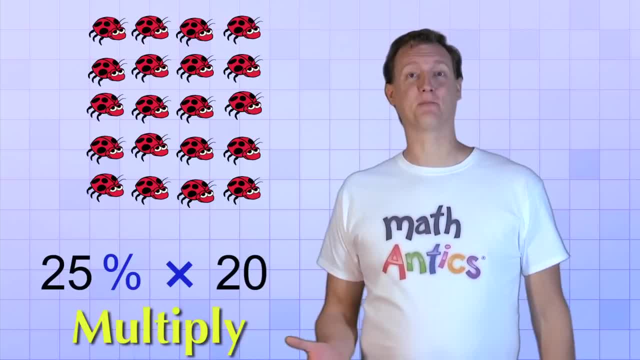 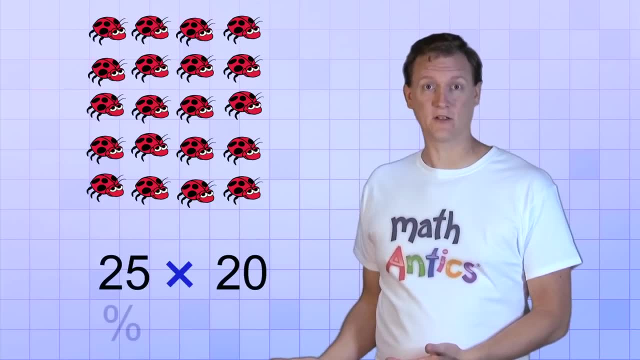 Great. So all we have to do to find a percent of a number is to multiply. But how do we multiply a percent and a number together? Do we just forget about the percent sign and multiply the numbers together? No, If we did it that way, our number would be WAY too big. 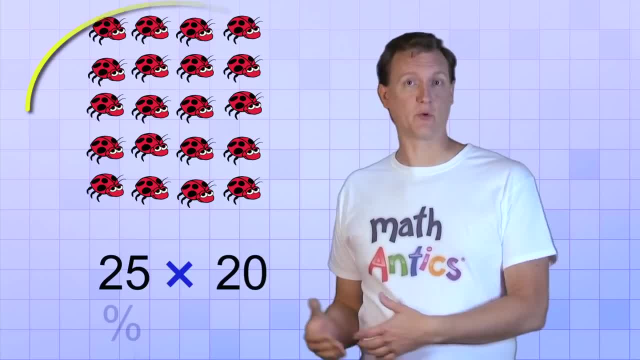 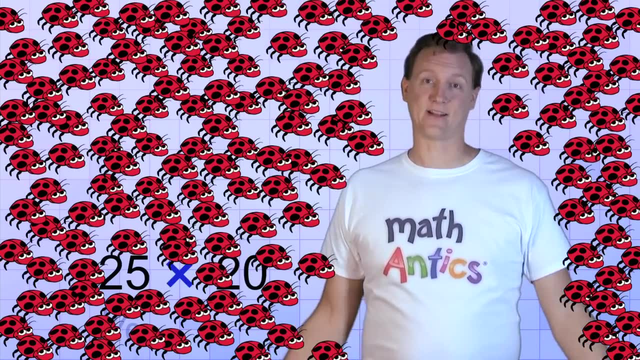 25% should be a smaller part or a fraction of 20 ladybugs. But if we did 25 times 20, we'd get 500 ladybugs. Clearly that's not the right answer. Here's what we have to do instead. 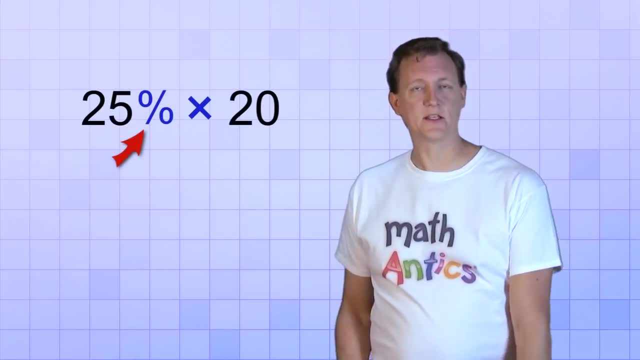 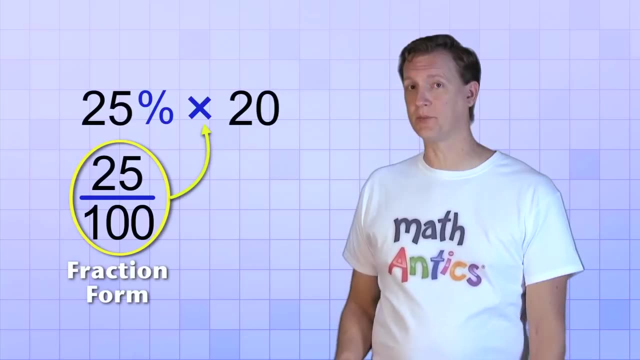 Remember that when you see a percent written like this with the percent sign, it's an abbreviation for a fraction, In this case 25 over 100.. So we need to use that fraction form when we multiply, since we're really multiplying by a fraction. 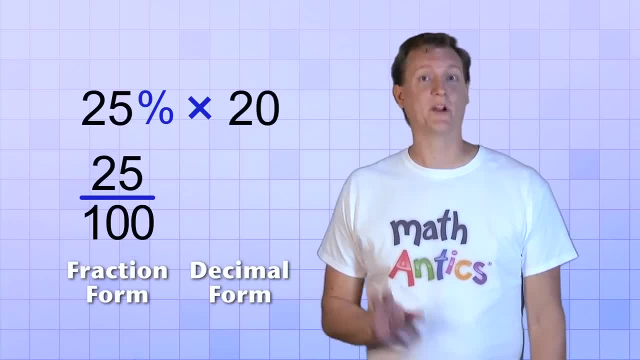 Now, some of you may also remember that percents have a decimal form. We'll get to that in just a minute. Okay then, if we use the fraction form of our percent, then our percent will be 25% over 100.. Okay then, if we use the fraction form of our percent, then our percent will be 25% over 100.. 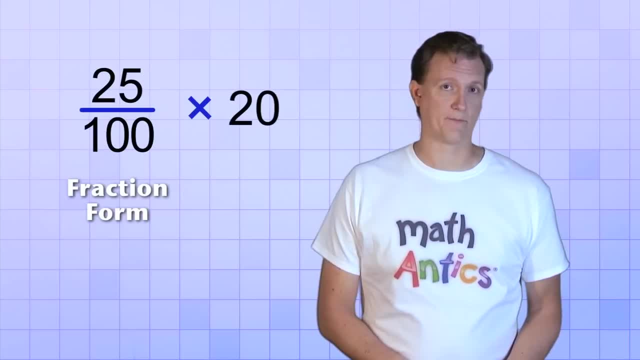 Okay, then if we use the fraction form of our percent, then our percent will be 25% over 100. Then our problem becomes 25 over 100 times 20.. Now that's a problem. we know how to do To multiply fractions. we just multiply the top numbers. 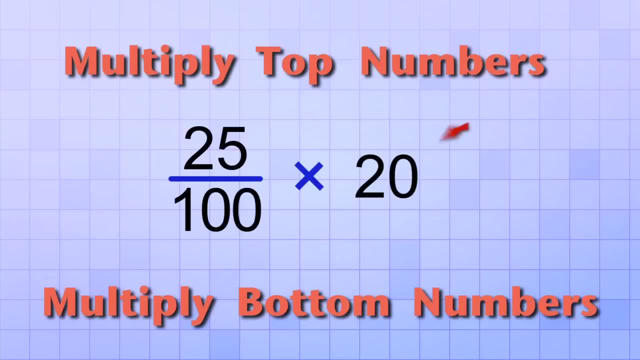 and then we multiply the bottom numbers to get the answer, And we can just write 20 as a fraction by putting 1 as the bottom number, because 20 over 1 is the exact same value as 20.. So let's go ahead and multiply. 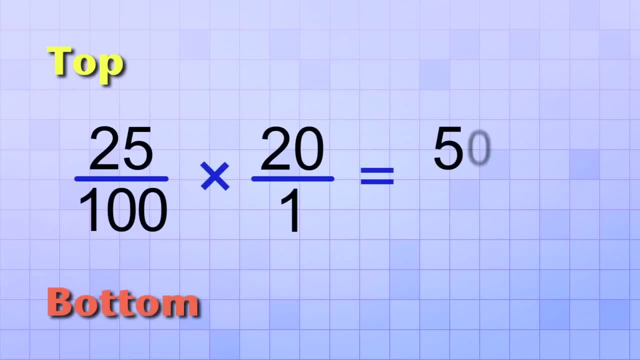 On the top we have 25 times 20,, which gives us 500. And on the bottom we have 100 times 1,, which is just 100. So our answer is 500 over 100.. Now, 500 over 100 might seem like a strange answer. 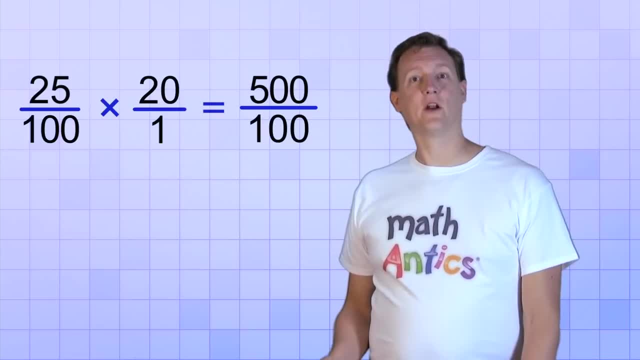 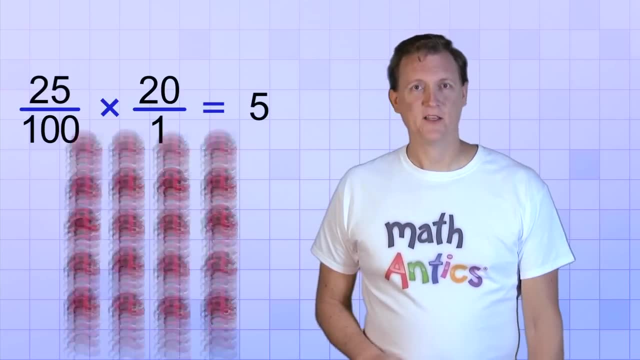 but that's just because we still need to simplify it. 500 over 100 simplifies to 5 over 1, and 5 over 1 is just 5.. That's much better. So 25% of 20 is 5.. 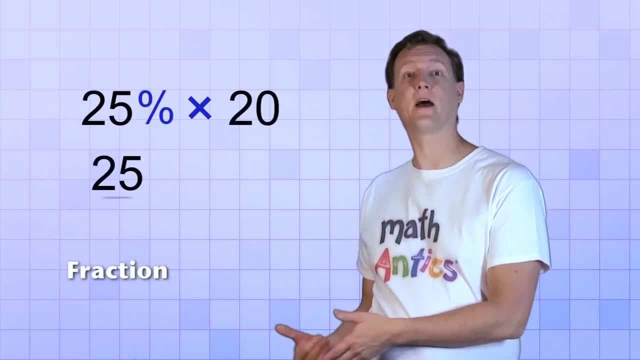 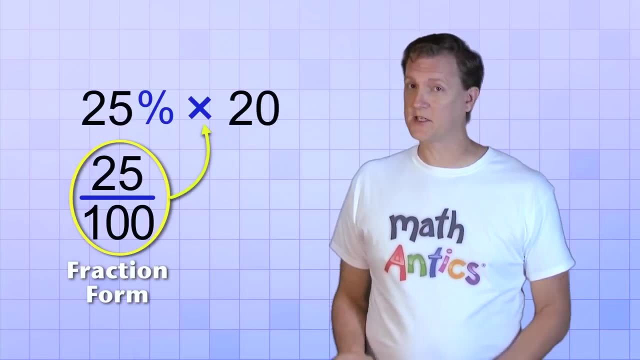 it's an abbreviation for a fraction, In this case 25 over 100.. So we need to use that fraction form when we multiply, since we're really multiplying by a fraction. Now, some of you may also remember that percents have a decimal form. 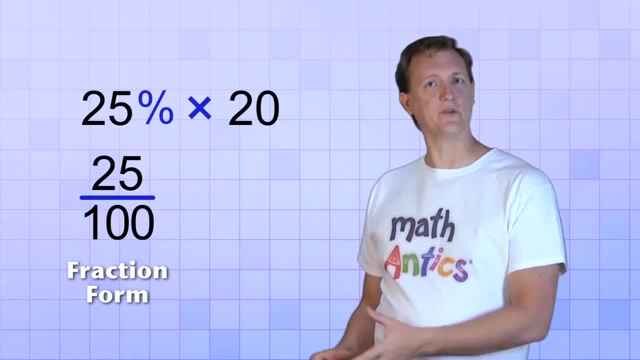 We'll get to that in just a minute. Okay, then, if we use the fraction form of our percent, then our problem is: Okay, then, if we use the fraction form of our percent, then our problem is: then our problem becomes 25 over 100 times 20.. 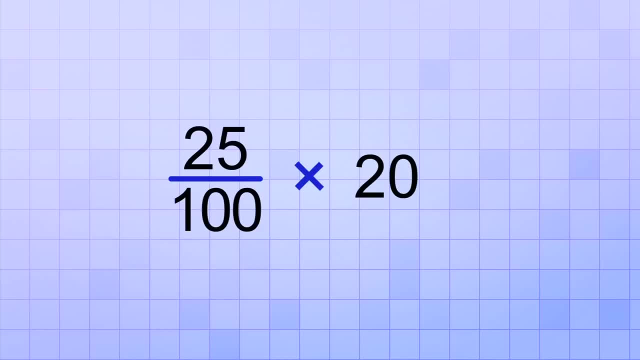 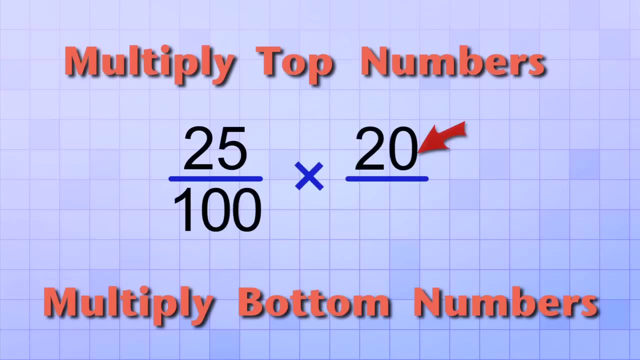 Now that's a problem. we know how to do To multiply fractions. we just multiply the top numbers and then we multiply the bottom numbers to get the answer, And we can just write 20 as a fraction by putting 1 as the bottom number. 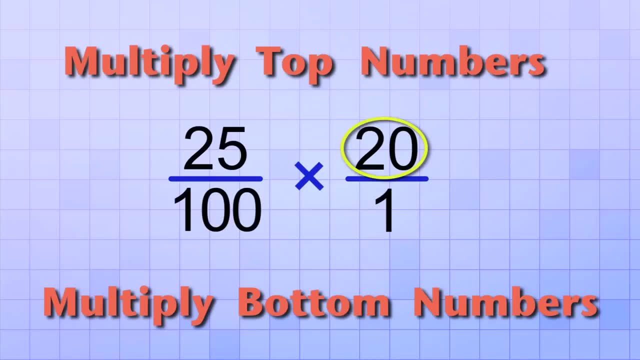 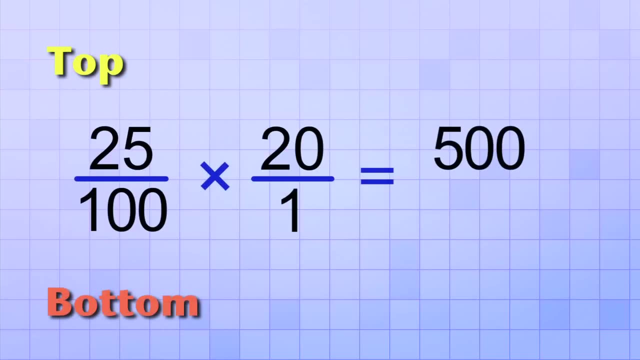 because 20 over 1 is the exact same value as 20.. So let's go ahead and multiply. On the top, we have 25 times 20,, which gives us 500.. And on the bottom, we have 100 times 1,, which gives us 100. 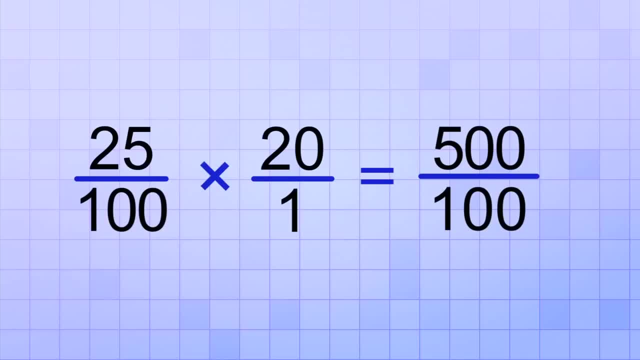 And on the bottom we have 100 times 1, which gives us 500.. And on the bottom we have 100 times 1, which gives us 100.. So our answer is 500 over 100.. Now, 500 over 100 might seem like a strange answer. 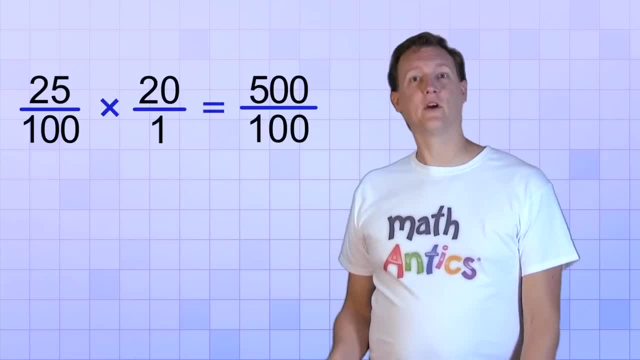 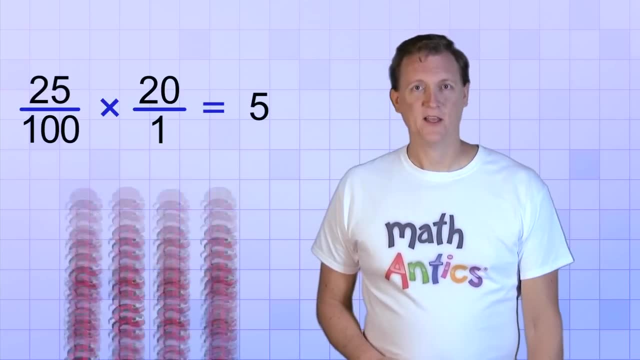 but that's just because we still need to simplify it. 500 over 100 simplifies to 5 over 1, and 5 over 1 is just 5.. That's much better. So 25% of 20 is 5.. 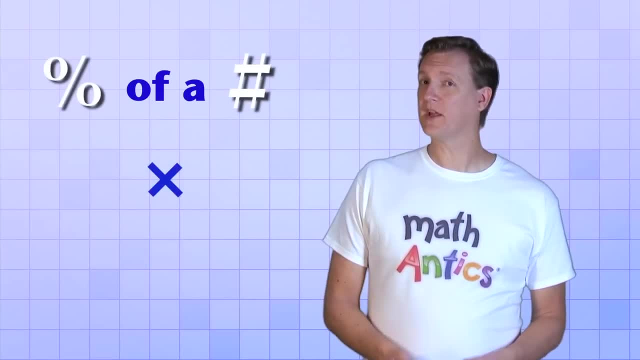 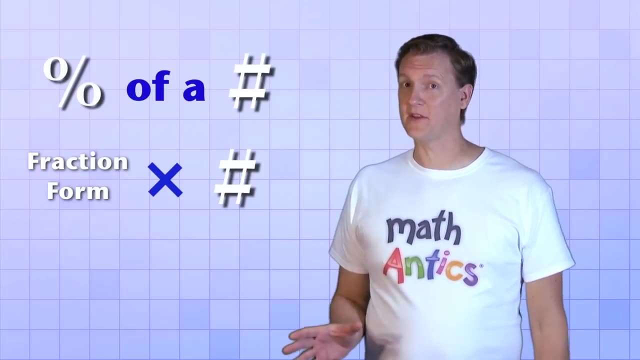 Alright. so to find a percent of a number, we just need to multiply the fraction form of the percent by the number and we have our answer. But there's another, slightly different method that you can use that works especially well if you're allowed to use a calculator. 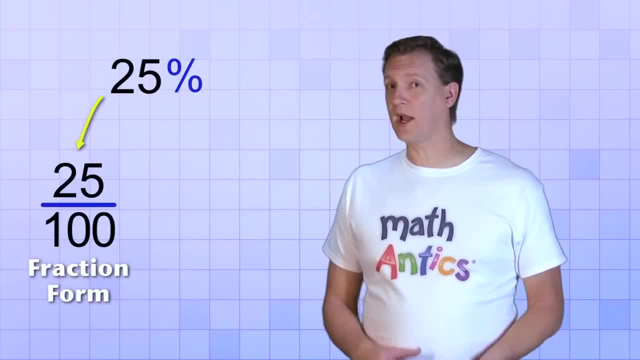 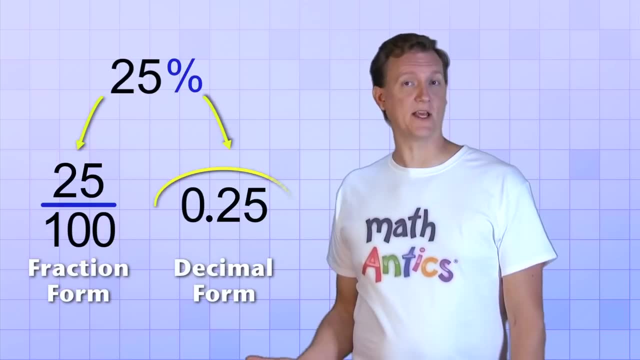 In our first percentages video, we learned that percents have both a fraction form and a decimal form. We've already seen how we can use the fraction form to find a percent of a number, but we can also use the decimal form if we want to instead. 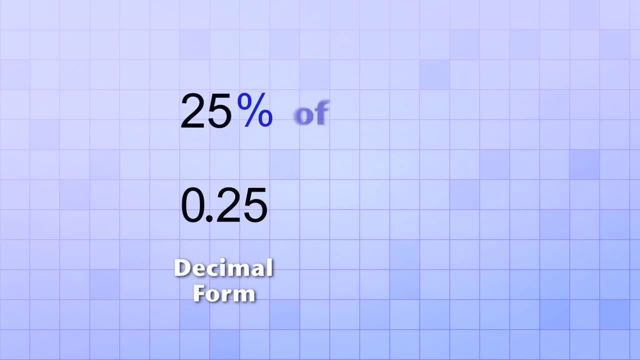 The procedure starts the same. If you need to find 25% of 20,, you first replace the word of with the multiplication symbol. Next we'll replace the percent, but with its decimal form. this time, 25% is the same as the decimal 0.25.. 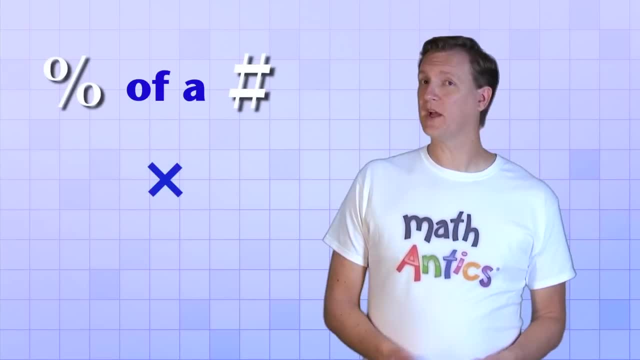 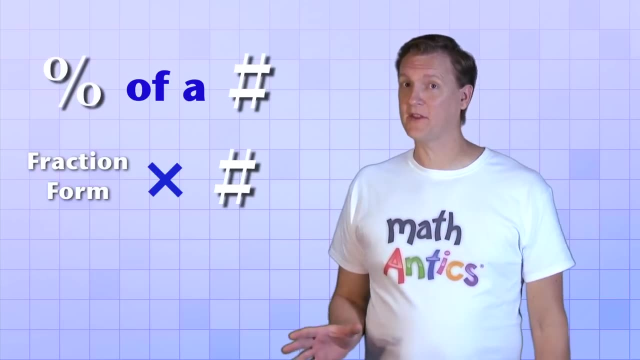 Alright. so to find a percent of a number, we just need to multiply the fraction form of the percent by the number and we have our answer. But there's another, slightly different method that you can use that works especially well if you're allowed to use a calculator. 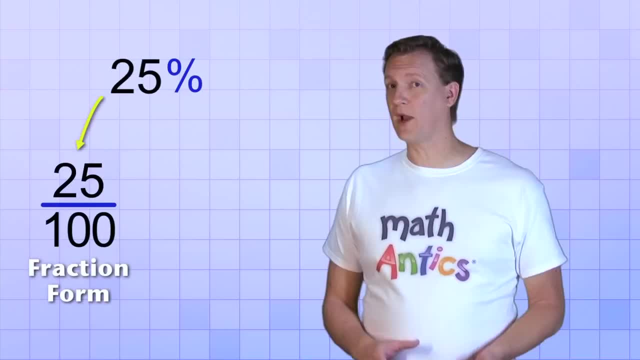 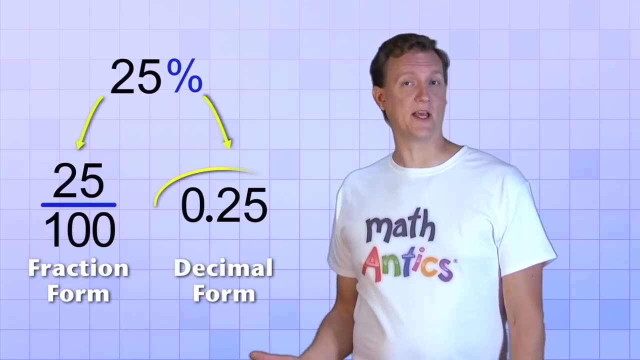 In our first percentages video, we learned that percents have both a fraction form and a decimal form. We've already seen how we can use the fraction form to find a percent of a number, but we can also use the decimal form if we want to instead. 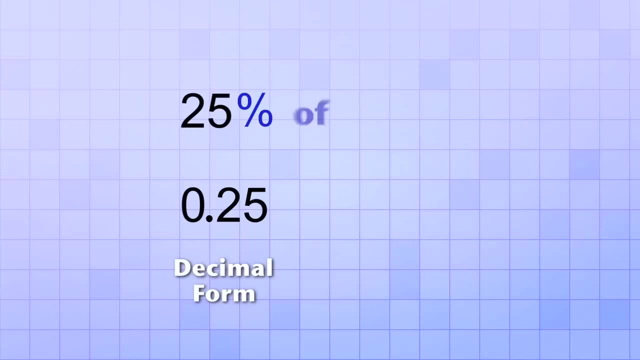 The procedure starts the same. If you need to find 25% of 20,, you first replace the word of with the multiplication sign. Next we'll replace the percent, but with its decimal form. this time, 25% is the same as the decimal 0.25.. 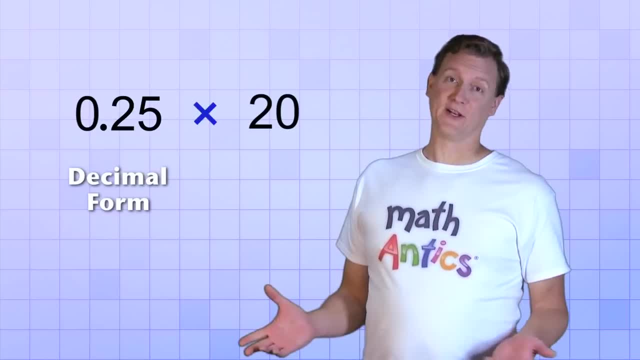 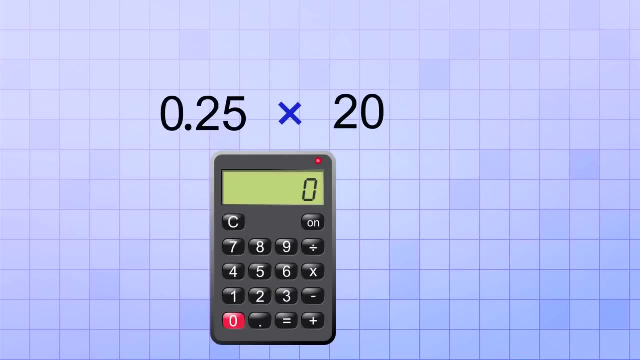 Then all we have to do is multiply, And although I could easily do the decimal multiplication by hand, I happen to have a calculator, so I'm going to use it. I just enter 0.25 times 20,, hit equals and I get 5.. 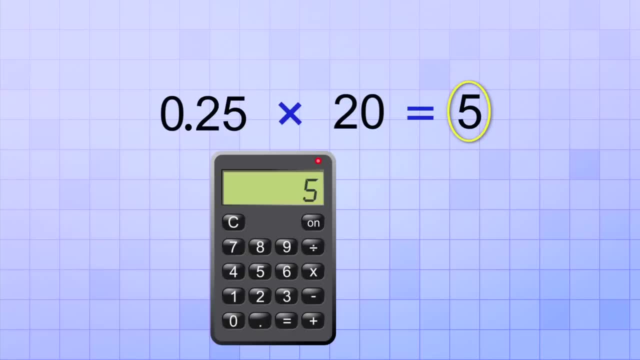 Yep, that's the same answer we got when we used the fraction form of 25%. Okay, that's the same answer we got when we used the fraction form of 25%. Okay, that's the same answer we got when we used the fraction form of 25%. 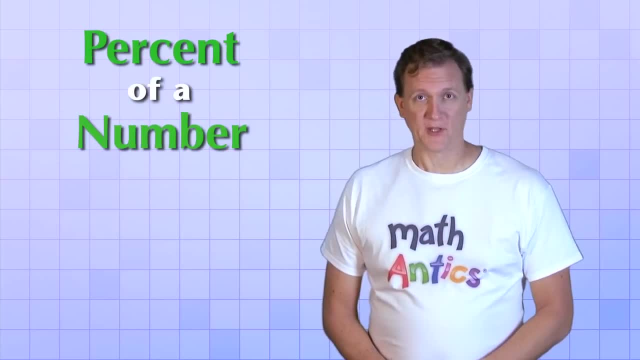 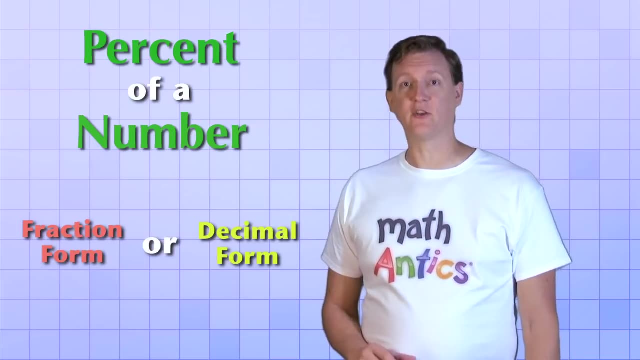 Oh yeah. So that's how you find a percent of a number. You just multiply the number by either the fraction form or the decimal form of the percent. Either way will give you the right answer, so you can choose whichever will be easier for you to do. 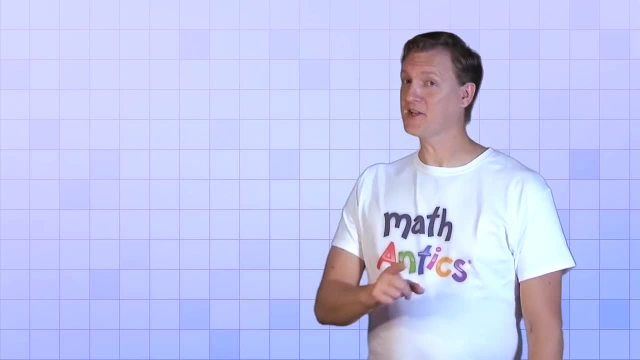 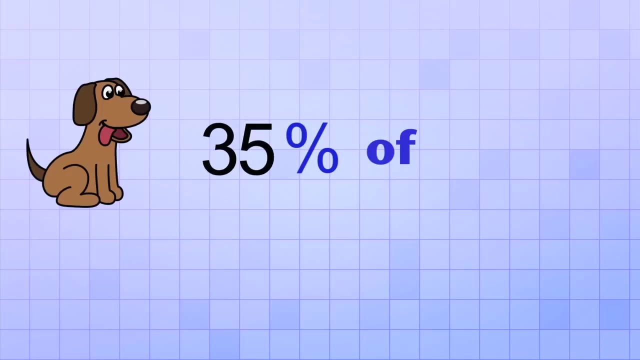 Let's see a couple more examples before you practice on your own. This next one involves money. Pretend that your best friend has a job walking dogs and offers to give you 35% of whatever he earns if you help him walk some of the dogs. 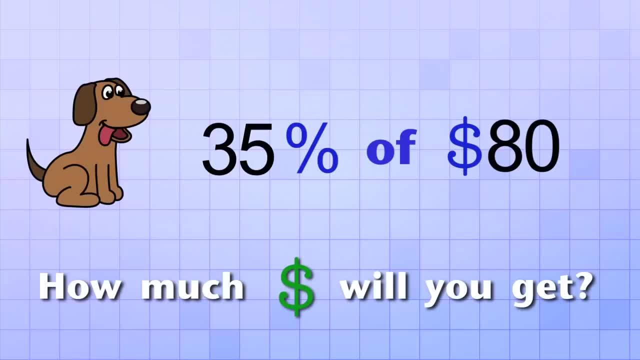 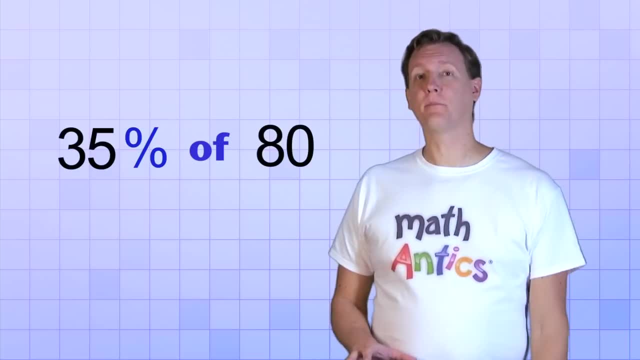 If your friend earns $80 that week, how much of the money will you get? In other words, you need to figure out what 35% of 80 is. Okay, then let's start by replacing the of with the time symbol. 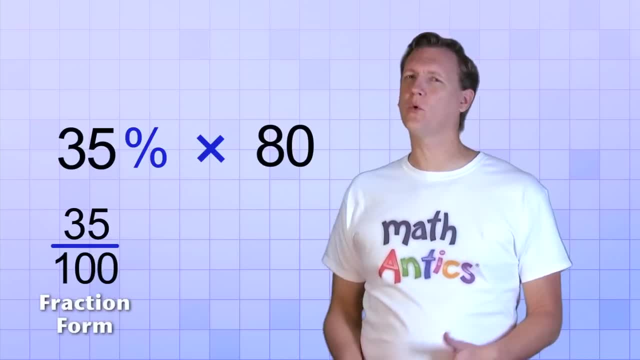 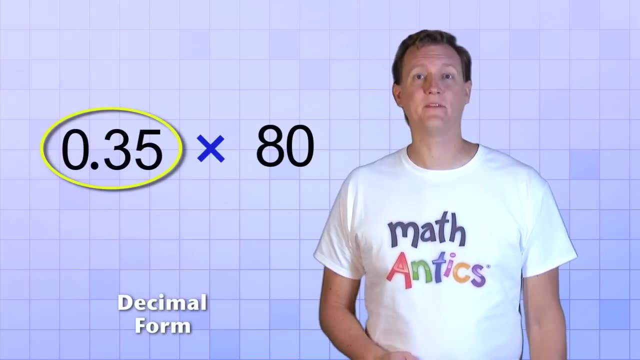 And next we have to decide if we want to replace the percent with its fraction form or its decimal form. I think I'll use the decimal form for this one, which means I'll replace the 35% with 0.35.. Now all we have to do is multiply 0.35 times 80,. 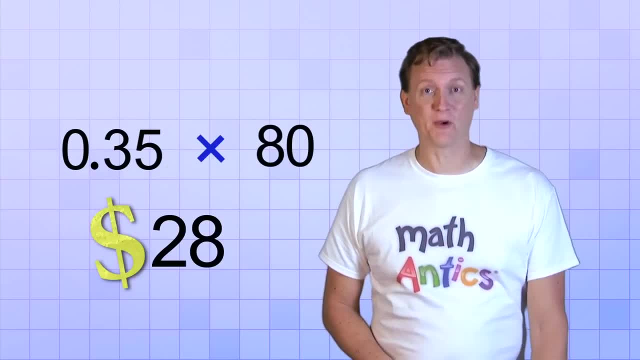 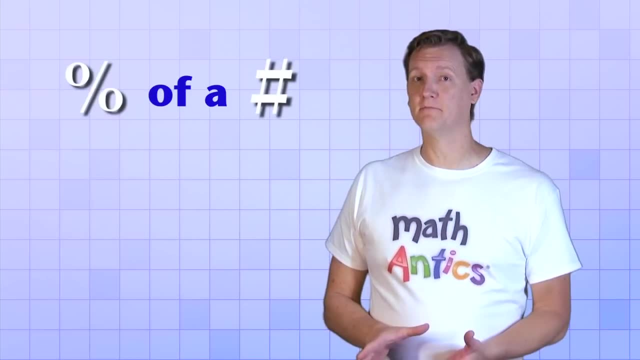 and that's 28.. That means you'll get $28.00 if you help your friend walk those dogs Cha-ching. Okay then, in the last two problems we found a percent of a number which, like we learned at the beginning of the video, 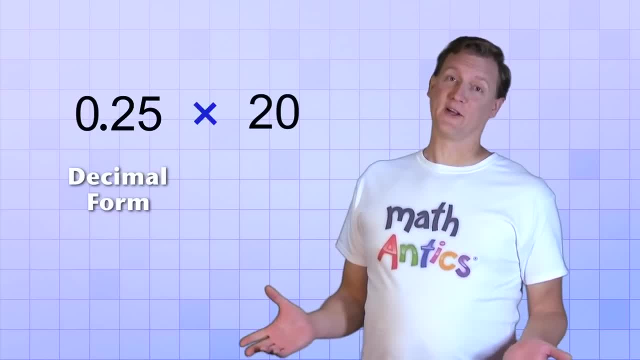 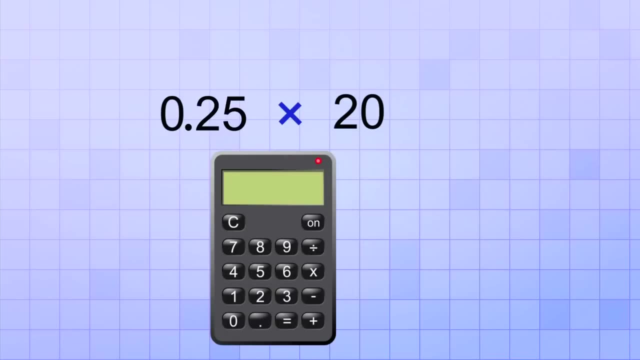 Then all we have to do is multiply, And although I could easily do the decimal multiplication by hand, I happen to have a calculator, so I'm going to use it. I just enter 0.25 times 20,, hit equals and I get 5.. 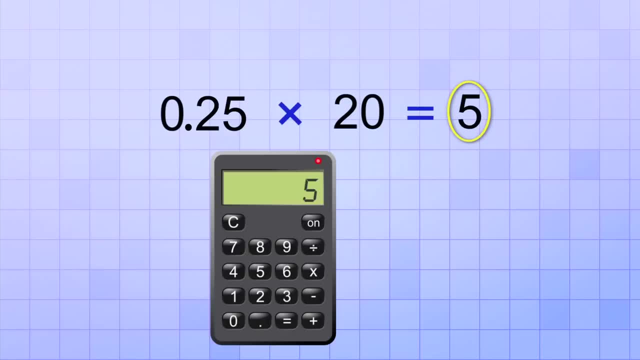 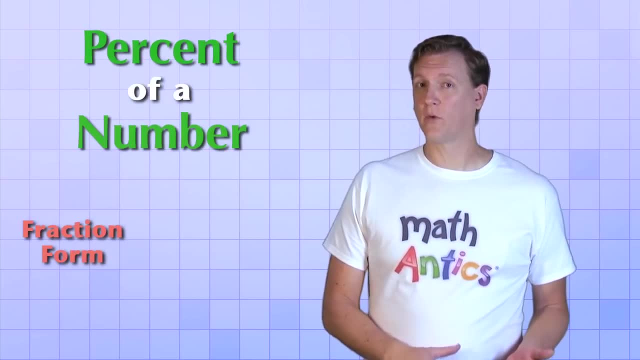 Yep, that's the same answer we got when we used the fraction form of 25%. Oh yeah, So that's how you find a percent of a number: You just multiply the number by either the fraction form or the decimal form of the percent. 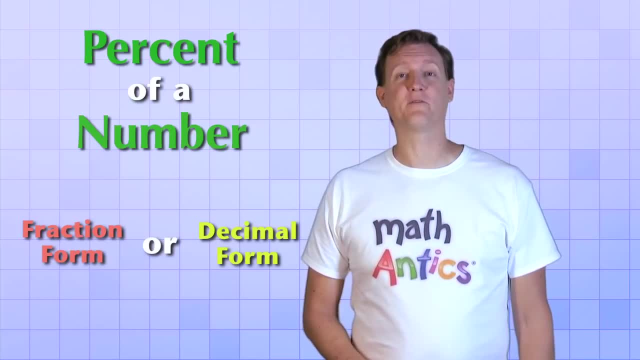 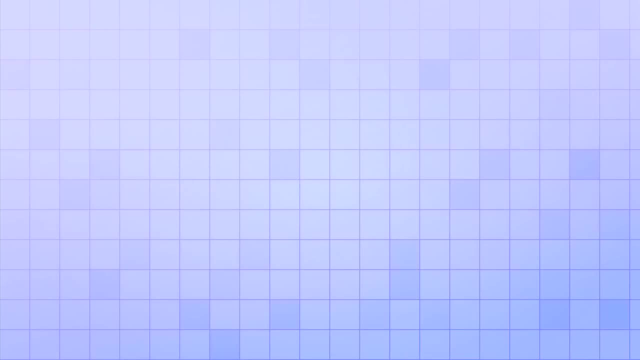 Either way will give you the right answer, so you can choose whichever will be easier for you to do. Let's see a couple more examples before you practice on your own. This next one involves money. Pretend that your best friend has a job walking dogs. 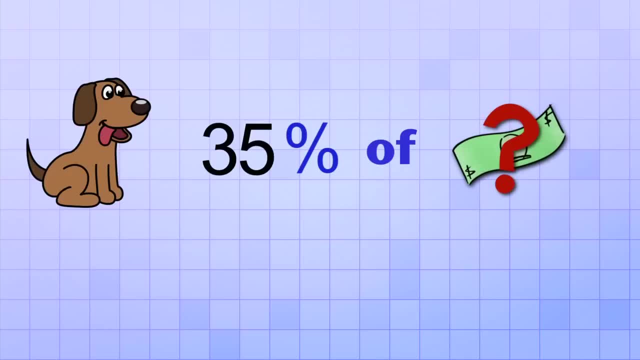 and offers to give you 35% of whatever he earns if you help him walk some of the dogs. If your friend earns $80 that week, how much of the money will you get? In other words, you need to figure out what 35% of 80 is. 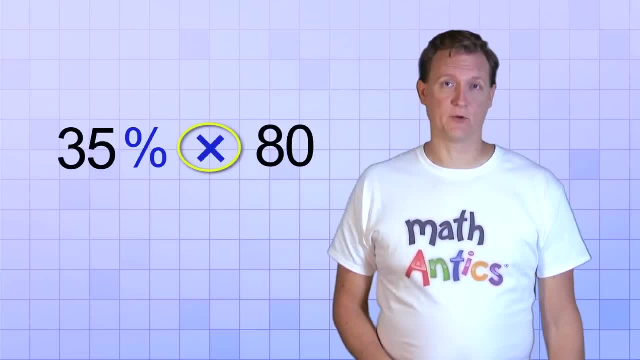 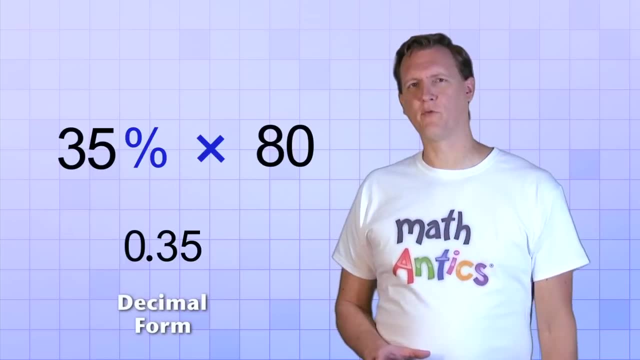 Okay, then let's start by replacing the of with the time symbol, And next we have to decide if we want to replace the percent with its fraction form or its decimal form. I think I'll use the decimal form for this one, which means I'll replace the 35% with 0.35.. 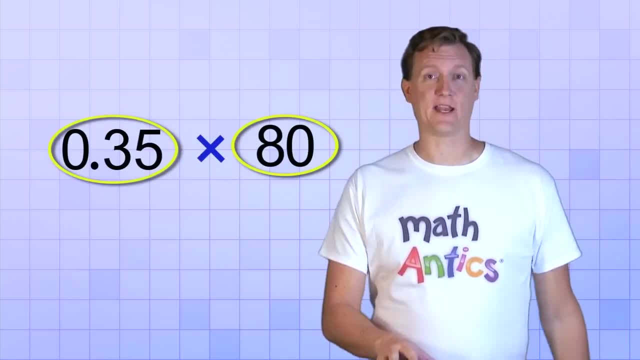 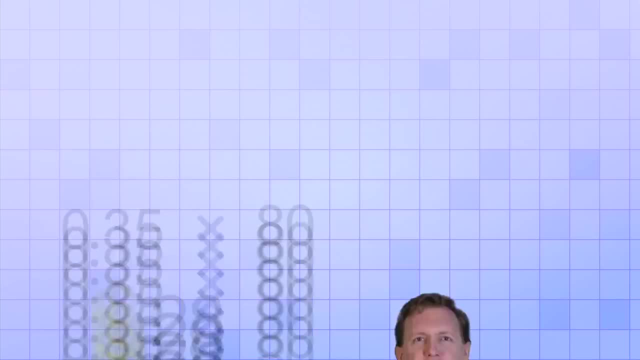 Now all we have to do is multiply 0.35 times 80. And that's 28.. That means you'll get $28.00.. If you help your friend walk those dogs Cha-ching, Okay. then in the last two problems we found a percent of a number. 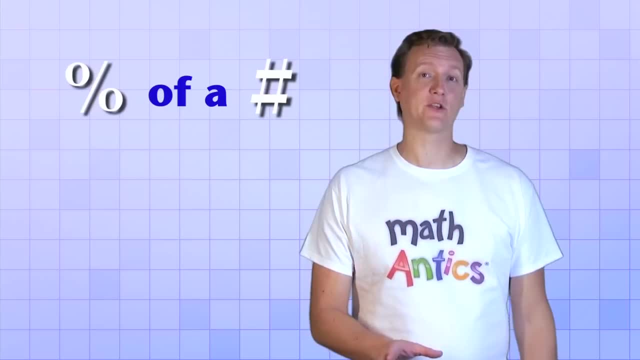 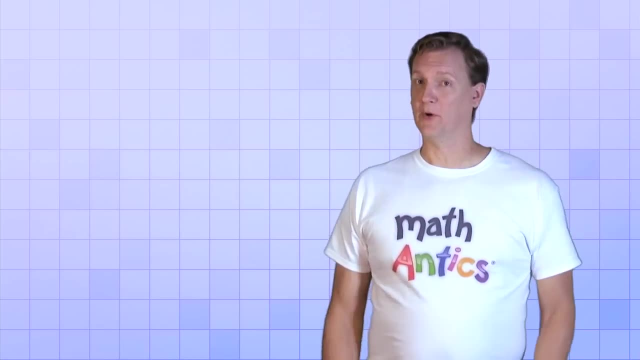 which, like we learned at the beginning of the video, just means finding a fraction of an amount And, like you'd expect when finding a fraction of something, the answer was smaller than the amount we started with. But remember, fractions can be improper too, which means that their value is greater than 1.. 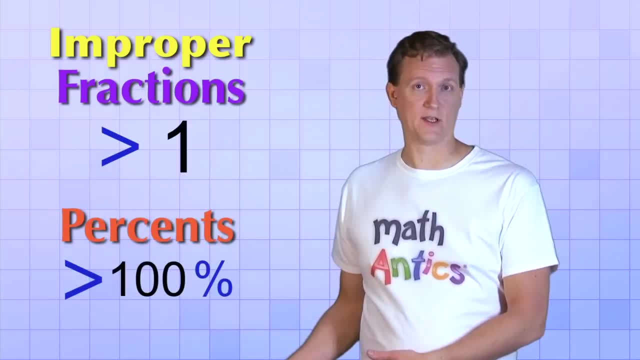 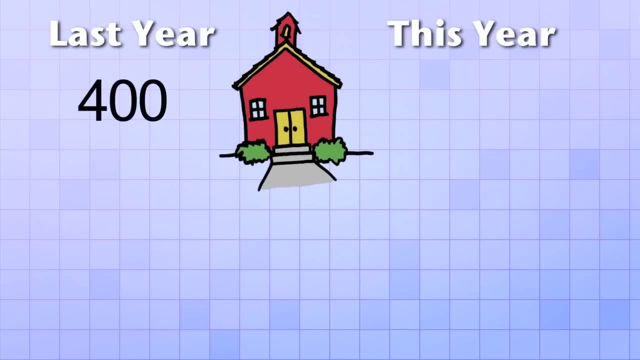 And, in the same way, percents can be greater than 100%. So you might come across situations like this: Suppose that last year your school had 400 students, but this year it has 120% of that amount. Well, 100% would mean the exact same number of students as last year.